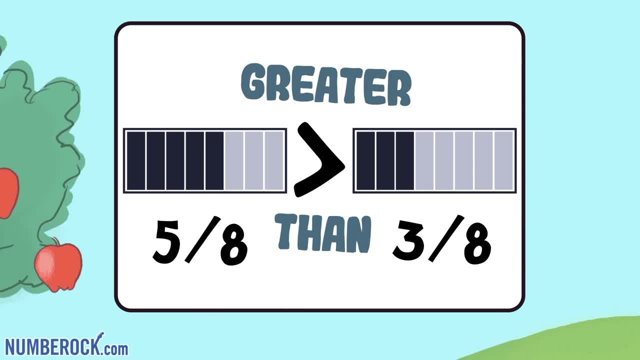 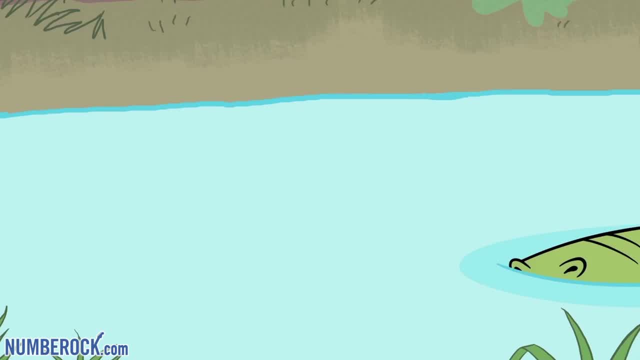 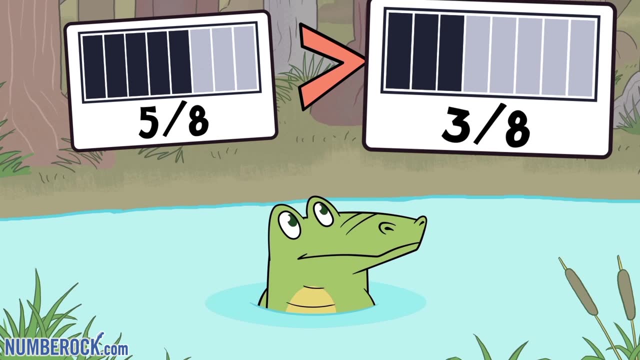 The equal parts for the gated is C. The 5-8 is greater than 3.. The equal parts for the gated is C: The fraction that is greater gets eaten by the alligator. The fraction that is least is never part of his feast. 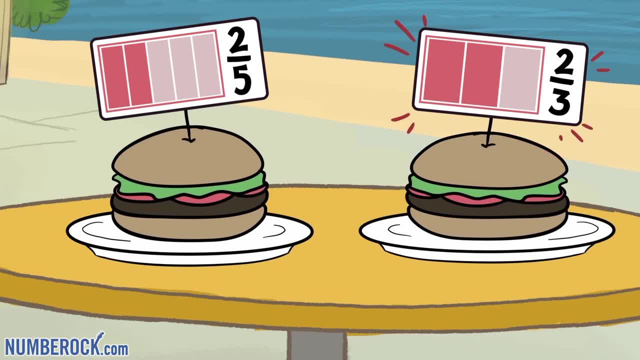 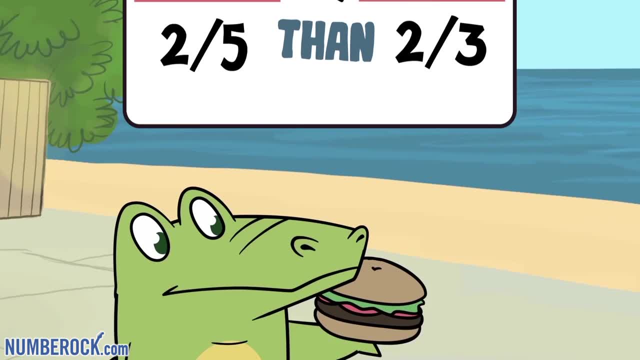 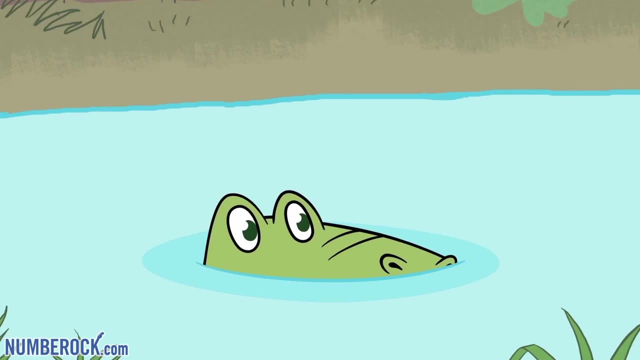 2-5 and 2-3, the greater faction is the one that he prefers. He imagines fraction bars on each side. 2-5 is less. he picks 2-3 and opens wide. The fraction that is greater gets eaten by the alligator. 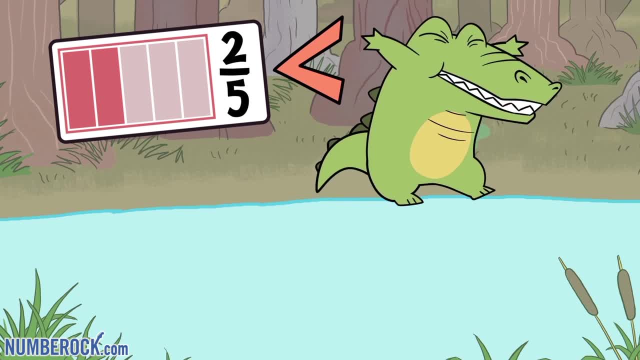 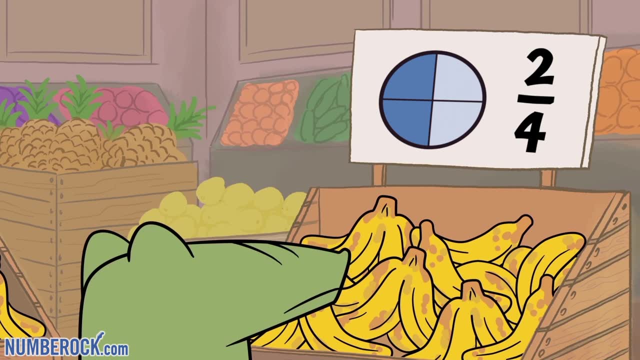 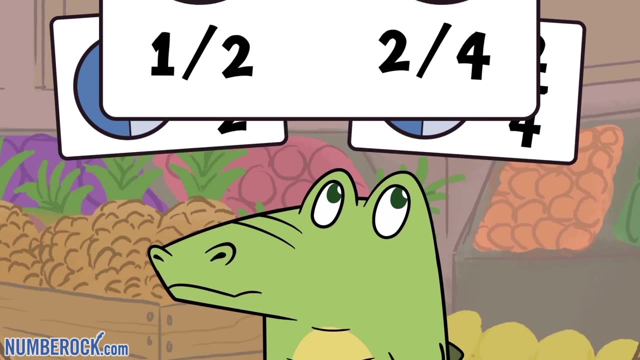 The fraction that is least is never part of his feast. Now, the values are the same on each side. The gator wants to eat, but he can't decide. One half on the left and two fourths on the right, The fractions are equivalent, so he takes a huge bite. 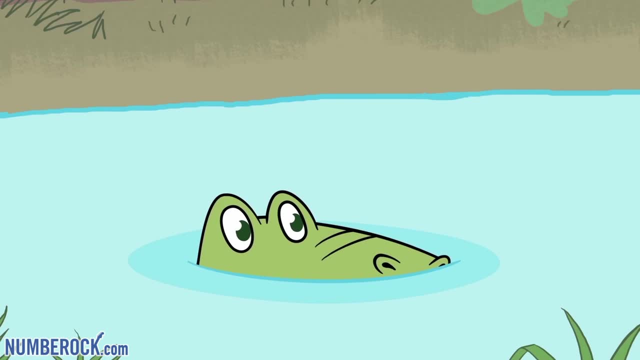 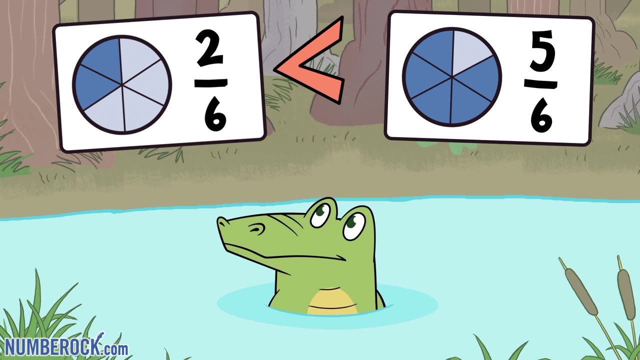 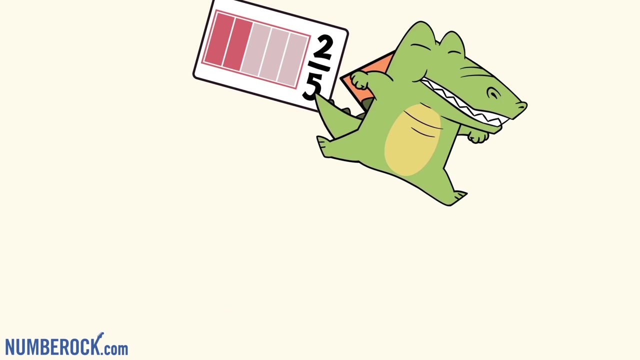 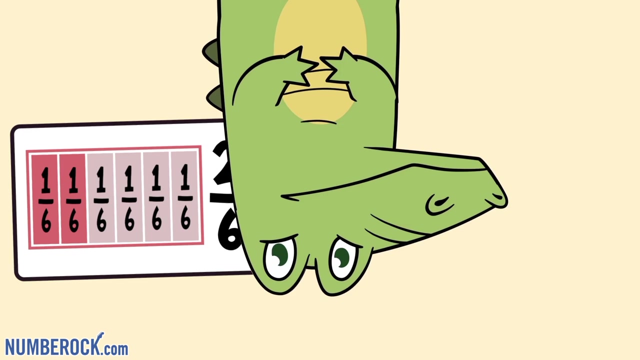 The fraction that is greater gets eaten by the alligator. The fraction that is least is never part of his feast. The fraction that is greater gets eaten by the alligator. The fraction that is least is never part of his feast If there's a line underneath for greater than sine. 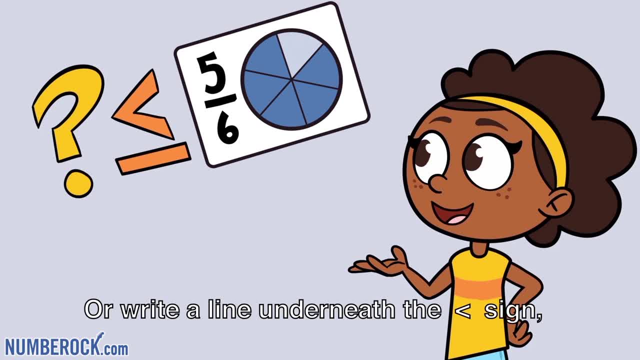 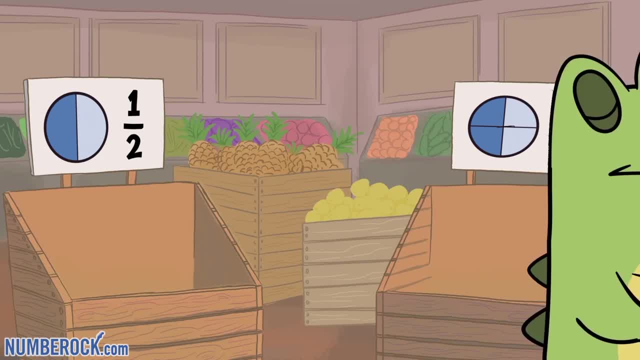 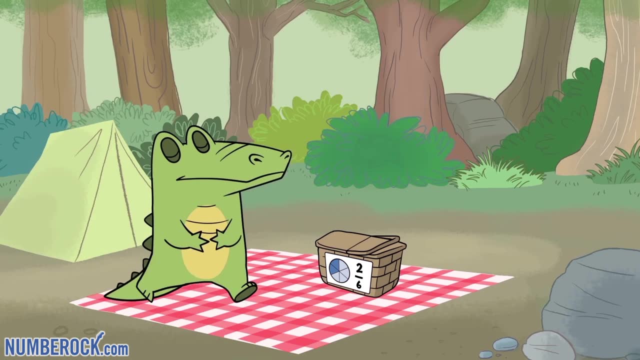 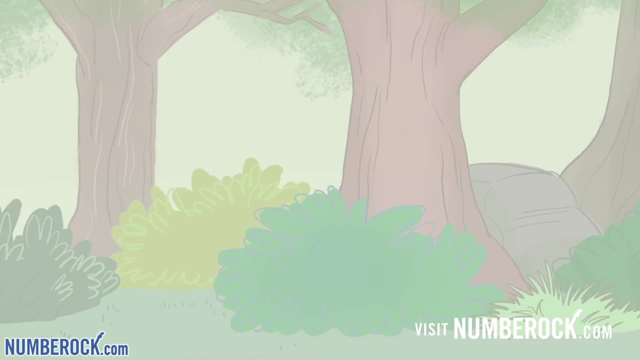 greater than or equal to is how the sine is defined. I'll write a line underneath the less than sign, and less than or equal to is the name of the design. Ooh Ooh Ooh, Hi there, I'm an alligator, so let's keep this snappy. 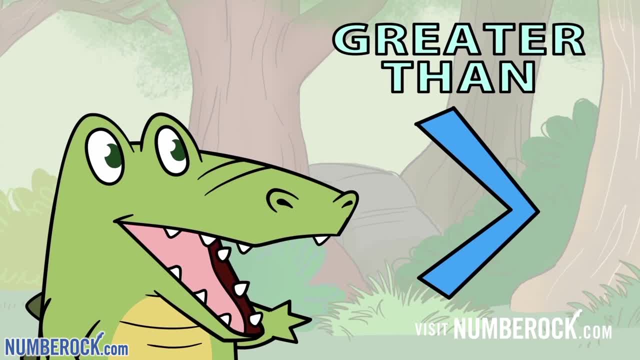 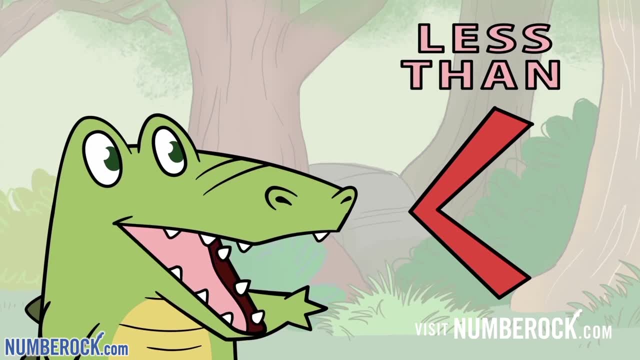 I'd like to take this opportunity to tell you that the greater than symbol goes from big to small, And it's called the greater than symbol. The less than symbol goes from small to big, And it's called the less than symbol. The larger fraction always goes on the open side of the angle.